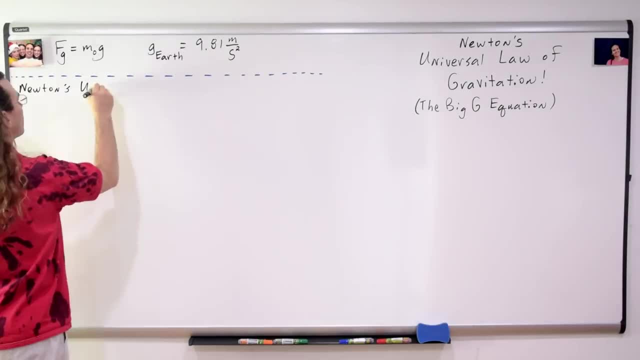 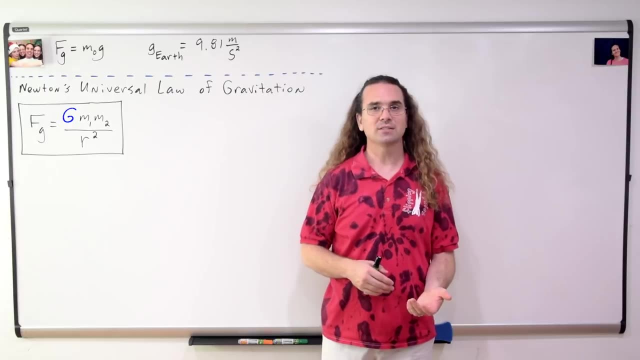 is Newton's Universal Law of Gravitation. Force of Gravity, Mr, And the equation is: the force of gravity equals big G, or the universal gravitational constant times the mass of object 1 times the mass of object 2, all divided by r squared. 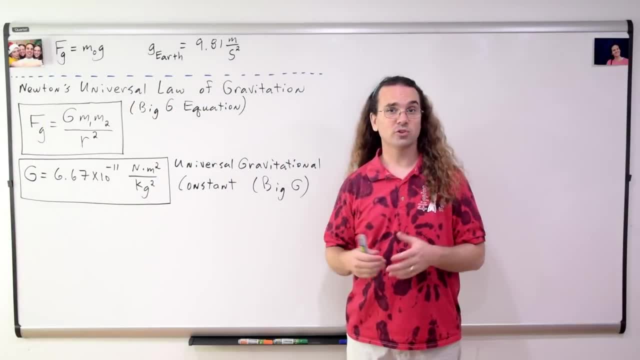 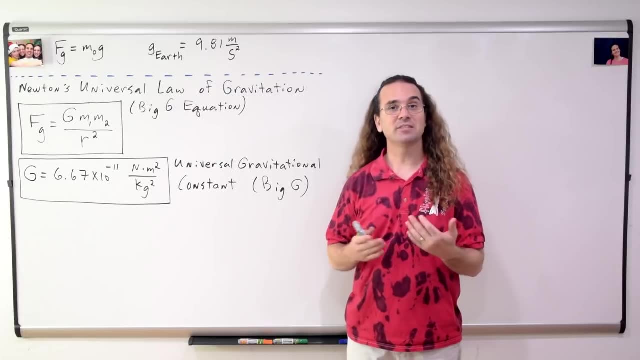 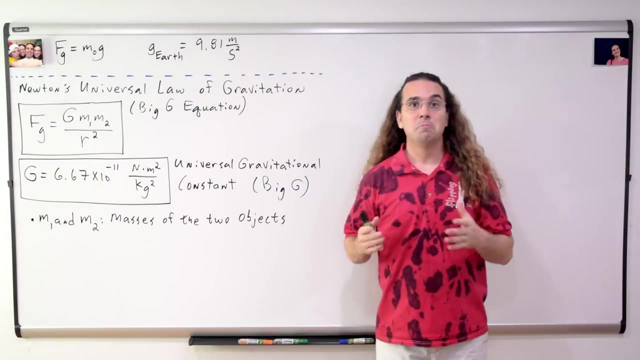 Big G, Mr. The universal gravitational constant, or big G as I like to call it, is an experimentally measured number and has an accepted value of 6.67 times 10 to the negative 11 newtons times meters squared over kilograms squared. 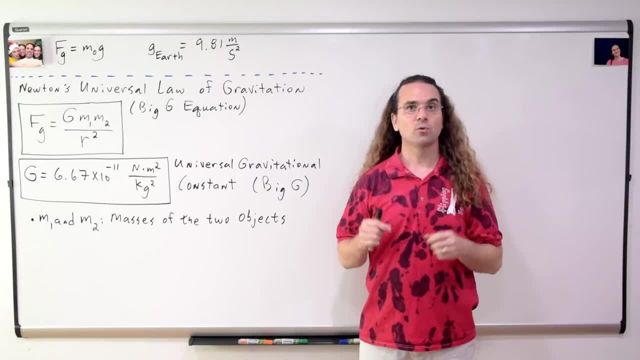 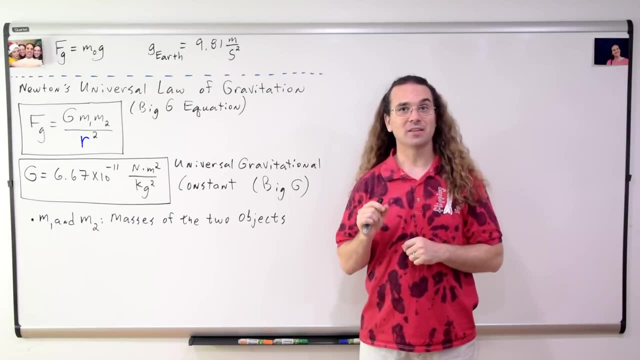 Mass 1 and mass 2 are the masses of the two objects which have the force of gravitational attraction between the two of them. And now let's talk about the r in this equation. Please class repeat after me: r is not the radius. 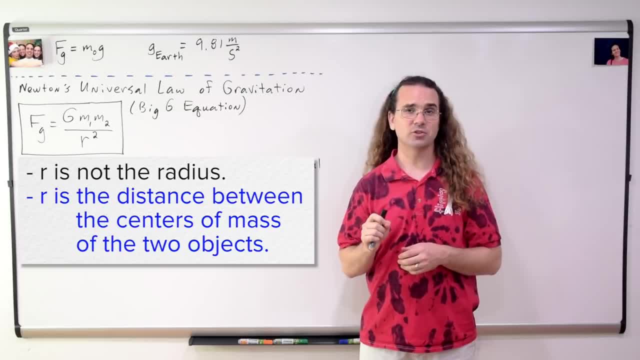 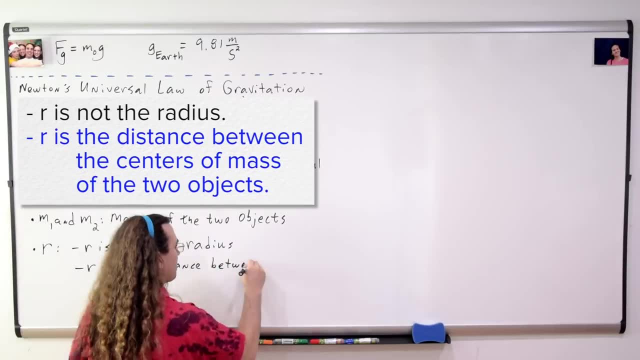 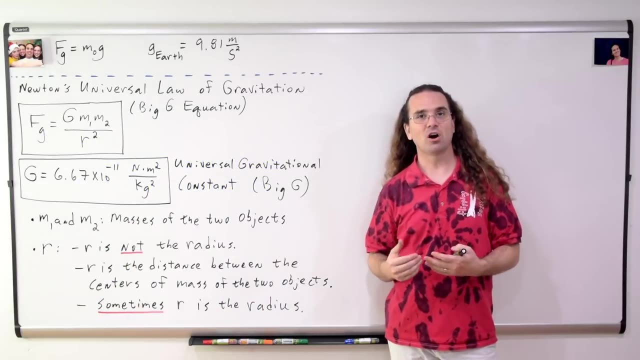 r is not the radius. r is the distance between the centers of mass of the two objects. r is the distance between the centers of mass of the two objects. So r is not defined as the radius. The definition of r is that it is the distance between the centers of mass of the two objects. 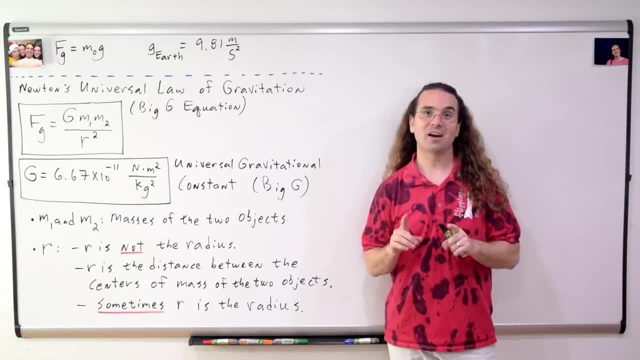 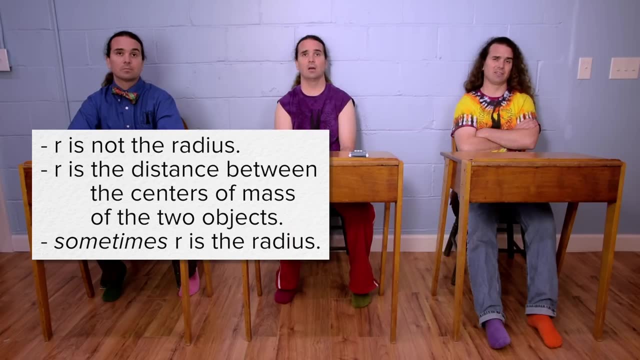 This can be confusing, because sometimes r actually works out to be the radius. However, r is not defined that way. r is not the radius, but sometimes it is the radius. Sure, r is not defined as the radius. However, there must be situations where r works out to be the radius. 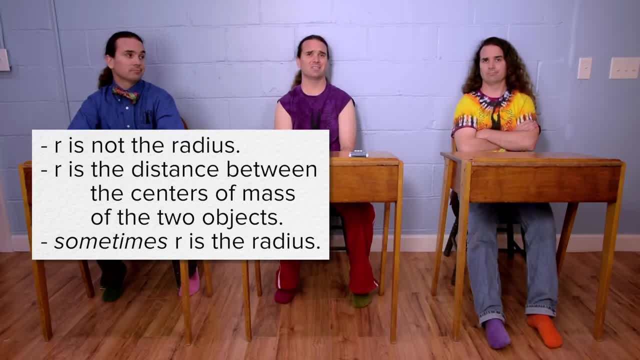 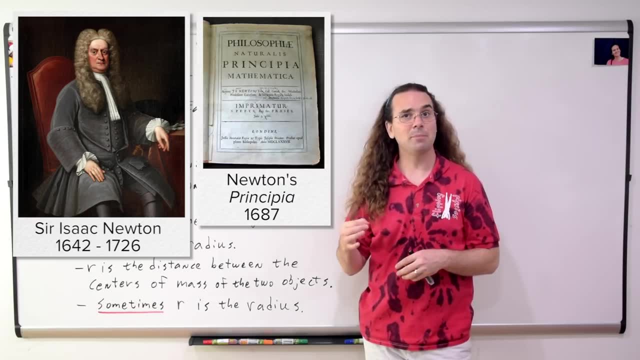 I wish they used a different letter for r, because that is confusing Me too. I totally agree. Just so you know, even though Sir Isaac Newton published his book Principia in 1687, which included his universal law of gravitation, Newton never actually was able to measure the radius. of the radius. 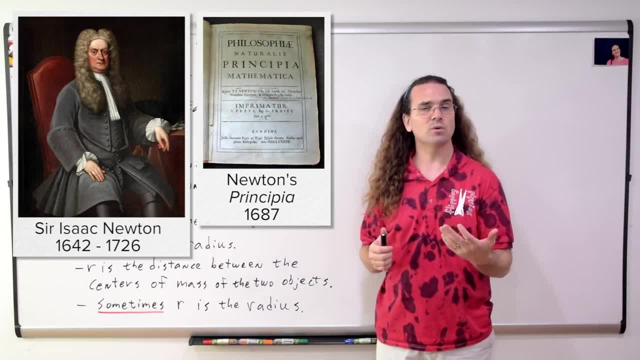 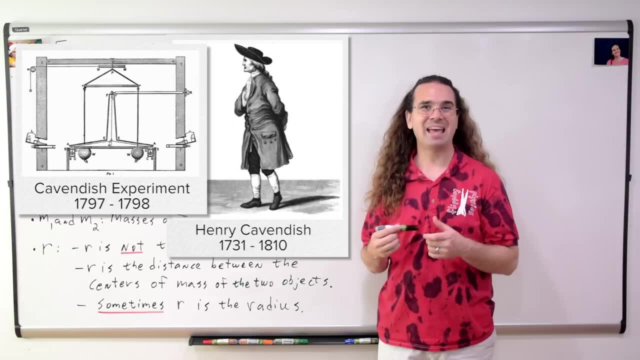 Newton never actually was able to measure the radius. of the radius He was able to measure the universal gravitational constant with any real accuracy. It wasn't until 1798, more than 100 years later, that a British scientist named Henry Cavendish performed the first accurate measurements. 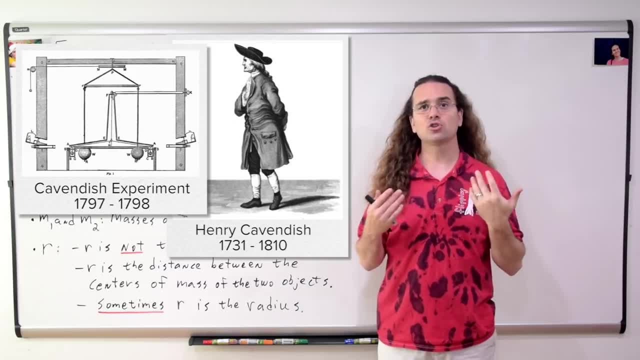 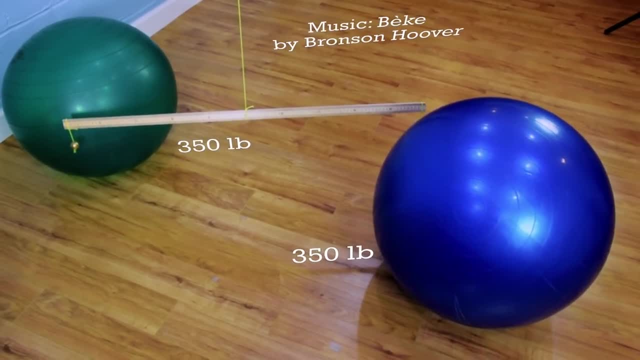 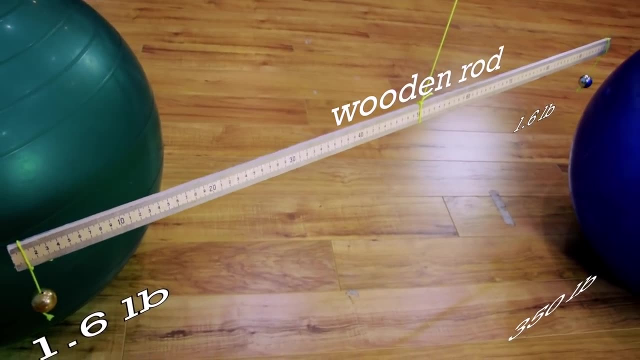 of the universal gravitational constant. He used a large torsion balance to measure big G. The torsion balance had two stationary 350-pound lead balls and, suspended on a metal wire, a 6-foot-long horizontal wooden rod with two 1.6-pound lead balls. 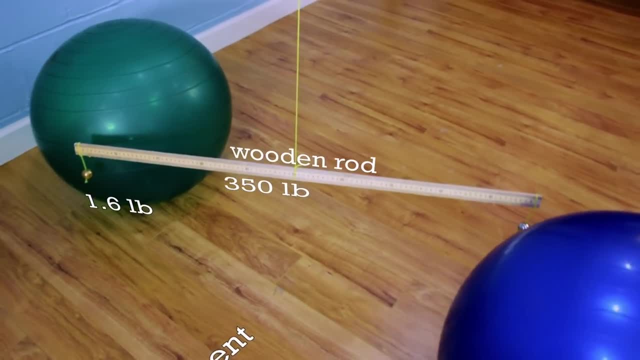 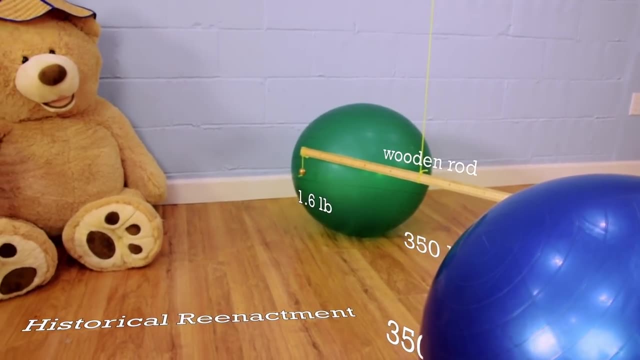 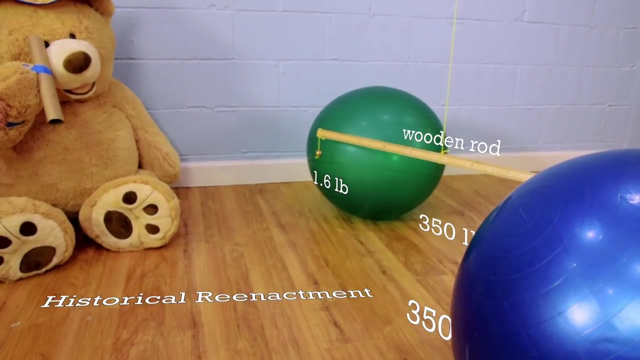 on either end of the wooden rod. The whole contraption was put in a large box and Henry Cavendish used telescopes to observe the slight motion of the two 1.6-pound lead balls toward the other 350-pound lead balls. You know what? 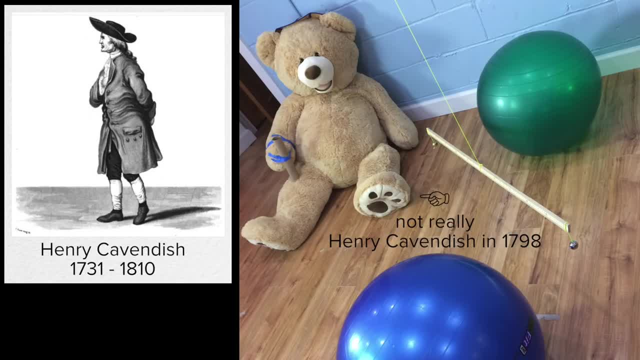 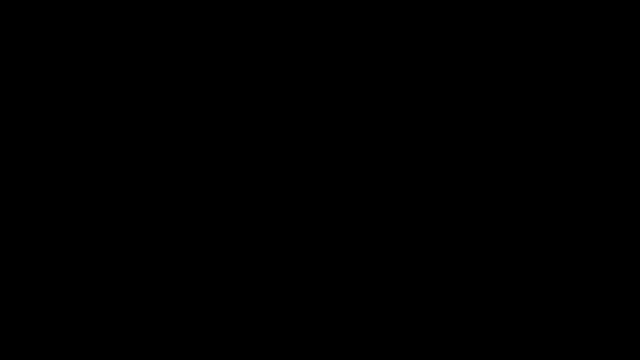 Let's talk through some qualitative examples of Newton's universal law of gravitation. Let's start with a completely empty universe. To be clear, right now, nothing exists in this universe. Now let's add one can of dog food, Notice, because there is only one object in this universe. 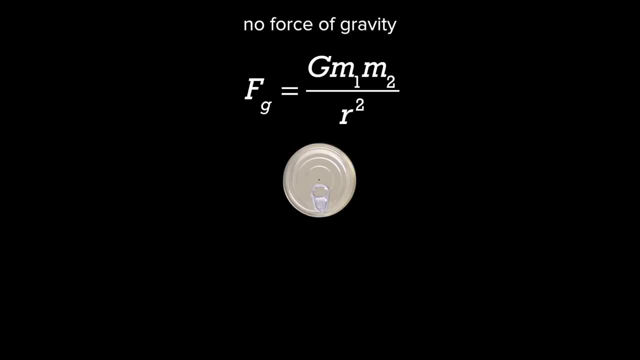 there is no force of gravitational attraction because it takes two objects- mass 1 and mass 2, to have a force of gravity. Without a second mass, there is no force of gravity. Now let's add a second can of dog food. 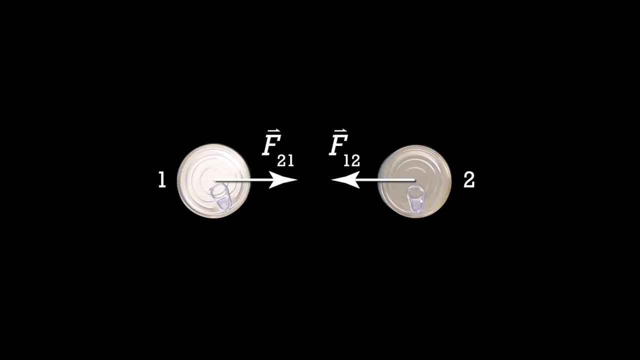 Notice. now, each of these cans of dog food has a force of gravitational attraction pulling it towards the other one. The force from can 1 on can 2 is the force of gravity. The force from can 1 on can 3 is the force of gravity. 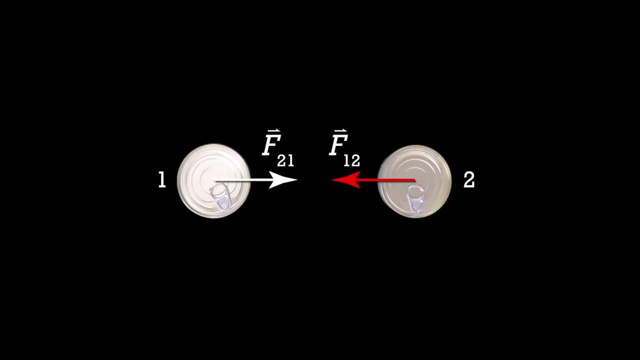 The force from can 2 on can 2 is pulling can 2 toward can 1.. And the force from can 2 on can 1 is pulling can 1 toward can 2.. Please realize: these two forces form a Newton's third law force pair. 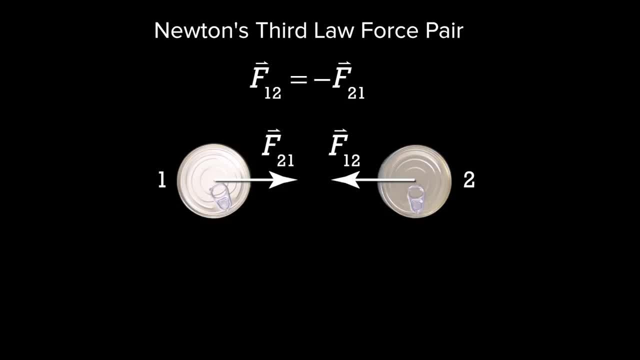 The force from can 1 on can 2 is equal and opposite to the force from can 2 on can 1.. If there is nothing else in this universe, wouldn't the two cans of dog food accelerate towards one another? Bo, that is a valid point. 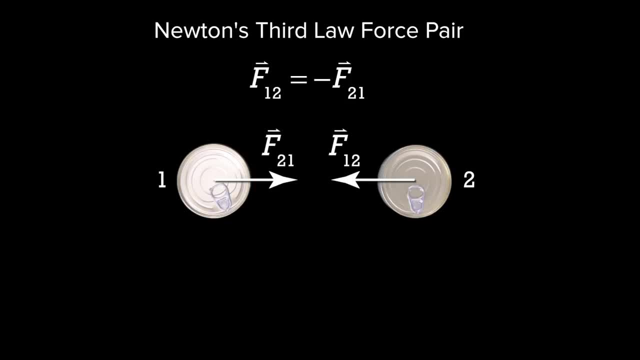 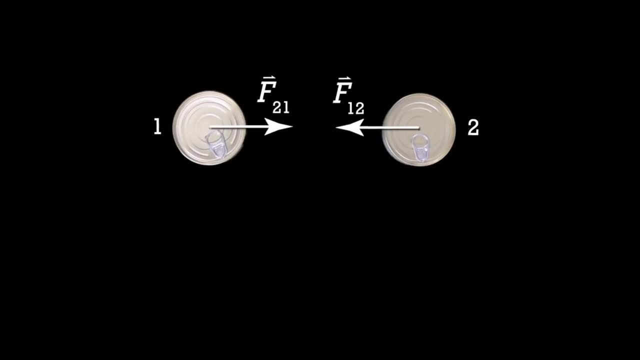 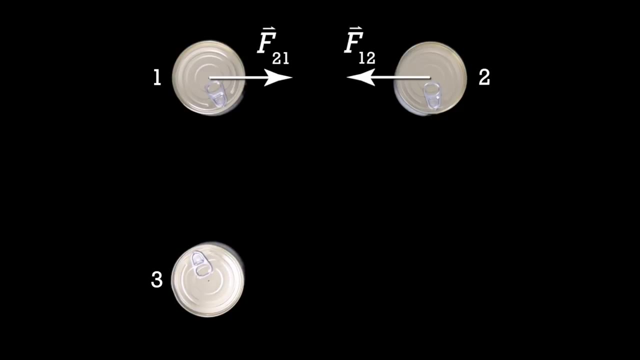 The cans would accelerate towards one another. However, right now I am just concerned about making sure you understand the forces, So let's not worry about the accelerations of the objects. Now let's add a third. can, Bobby, what additional gravitational forces exist in this universe? 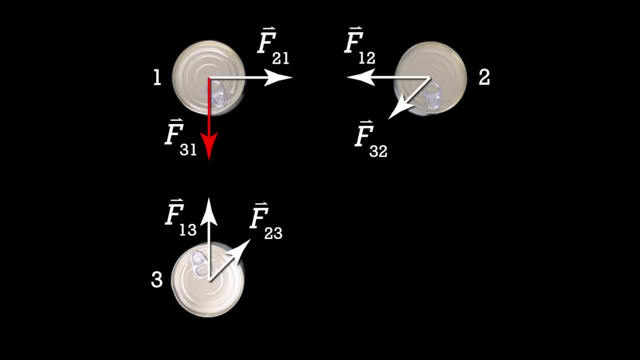 Well, can 1 is pulled toward can 3, and can 3 is pulled toward can 1.. Oh, and can 2 is pulled toward can 3, and can 3 is pulled toward can 4.. And can 3 is pulled toward can 2..